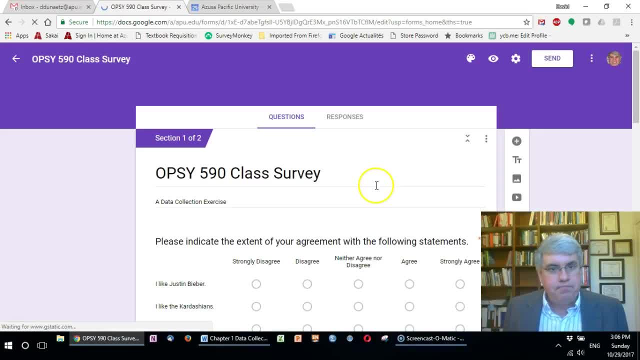 we click on our survey and it shows up the questions. We want the responses, So you go to responses. Once you've collected all that, you're going to now. this says that there was just one. you probably want at least 100, maybe up to 300,. 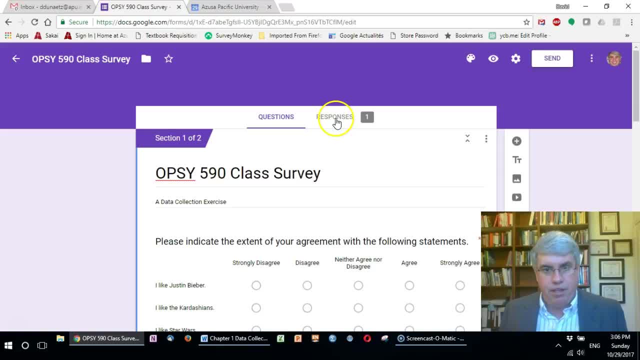 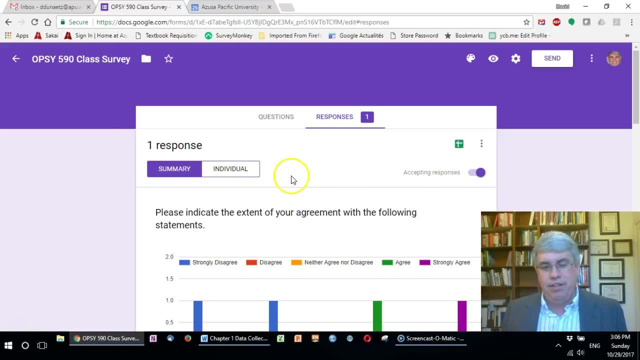 depending on the power that you have in your research design. We go over to responses and it says summary, individual. Now those don't really count. We want line by line. so we need to go to this green, cross over here and view the responses. 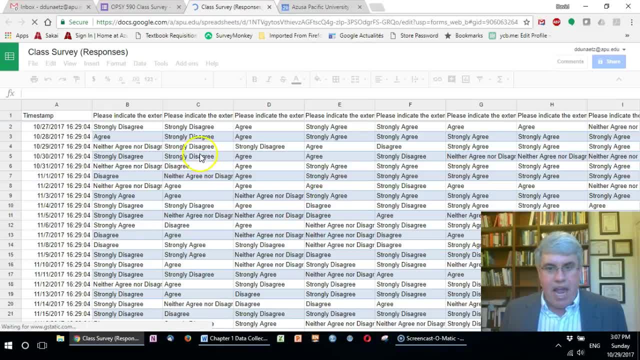 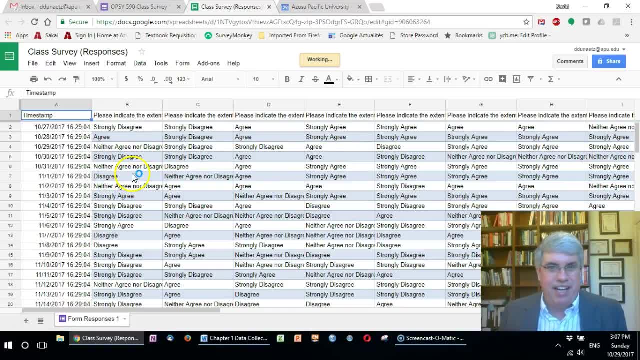 there's more than one piece of data that's collected, because I put other data into this, And what we want to do is we want to download this into Excel, because Google Sheets is good, but it's not nearly as powerful as Excel. 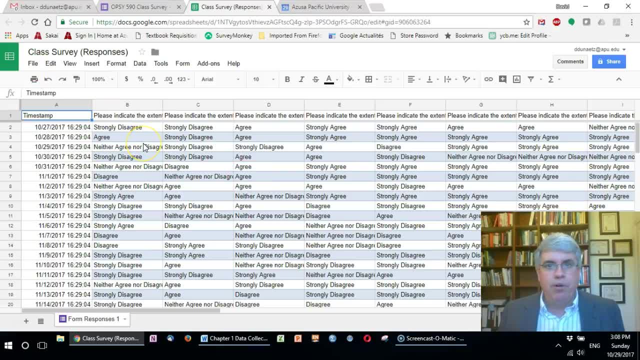 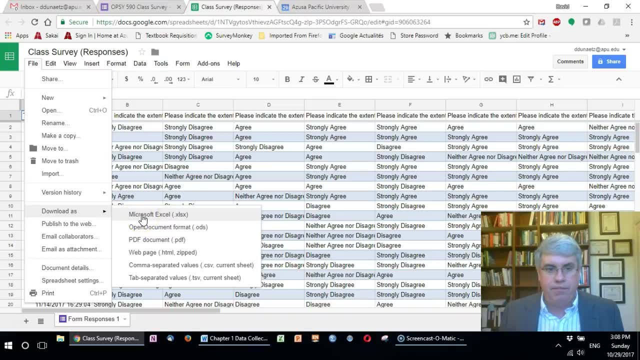 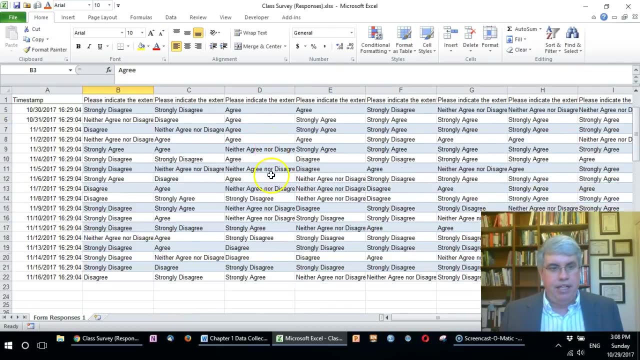 especially for statistical analysis. So I'm going to go over to File and I'm going to go to download as a Microsoft Excel file. Click on that. That opens up Excel and that gives me the data in Excel format. Now we want to do a number of things to this before we. 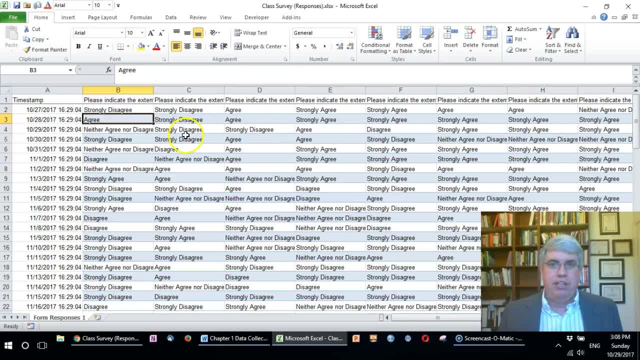 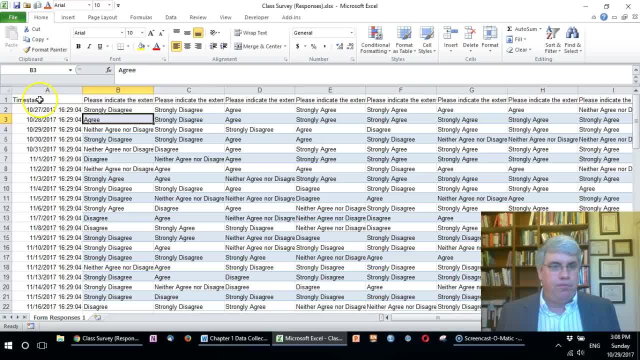 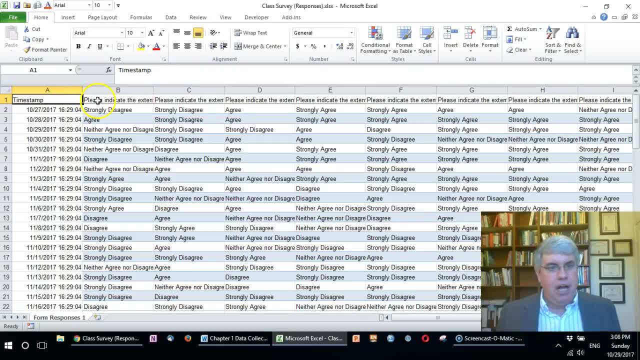 somebody the time and date that people filled in the form Over here we have the different items that were on Google surveys. Please indicate the extent of your agreement with the following statements: I like Justin Bieber: This one's. I like the Kardashians: This I like. 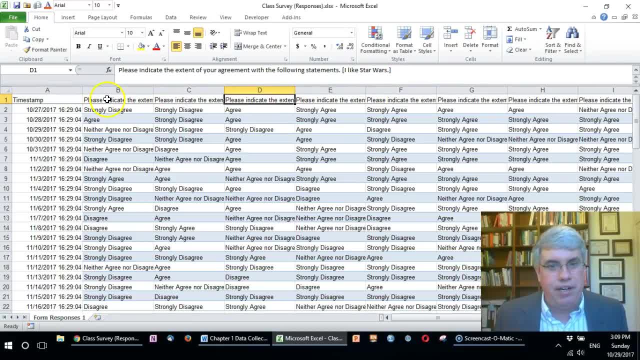 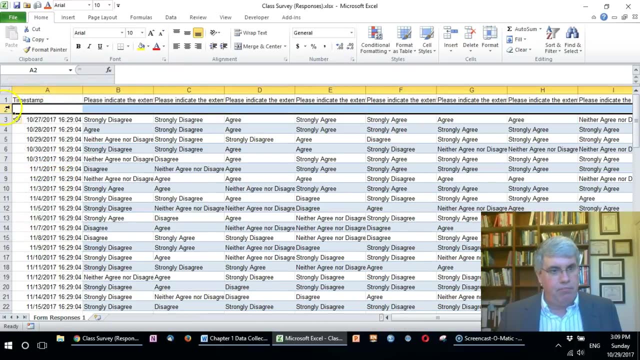 Star Wars. So these are real good variable names. What we need to do, first thing we're going to do, the first thing I like to do, is insert a couple blank lines at the top so that we can put in variable names. So I'm going to right click here and I'm going to press insert. That gives me one. 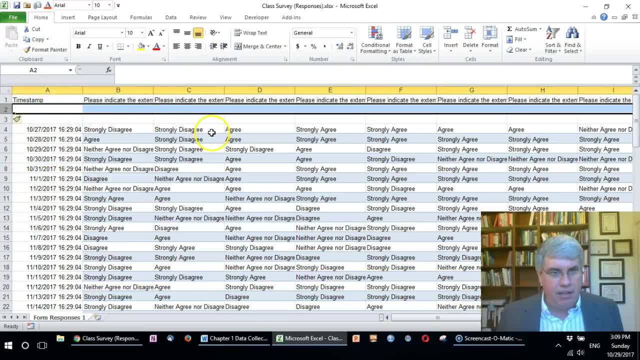 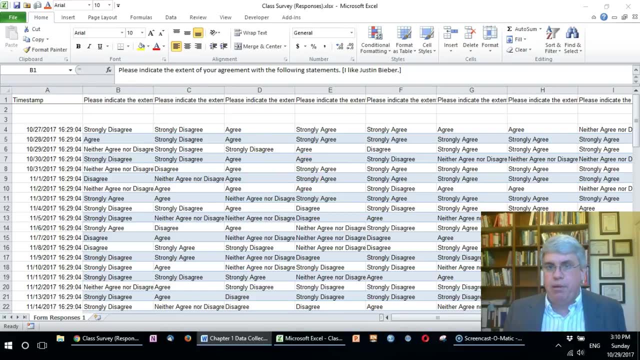 blank line And I'm going to insert a second blank line. Now in this line 3, I'm going to put different variable names. What variable names am I going to use? I'm going to use the variable names that I've prepared on what's known as the code books. Let me bring this over. 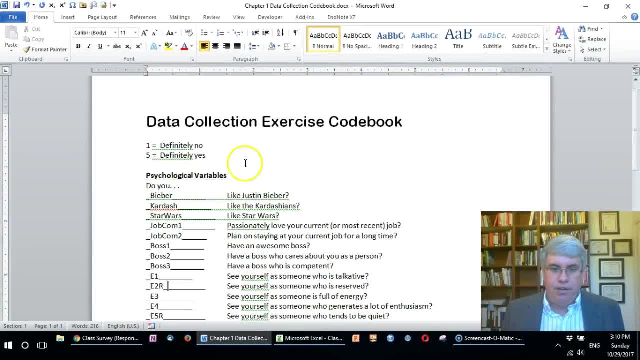 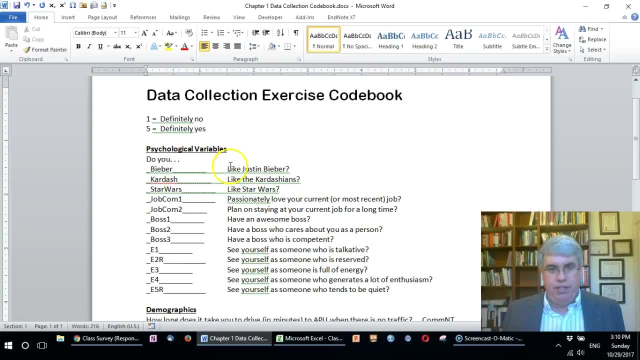 Here And this data collection code book that I have is I've got all the questions that I asked and I've given each question a name. It's like the question about how much you like Justin Bieber. I called it Bieber the Kardashians. I called the question about the Kardashians This question. 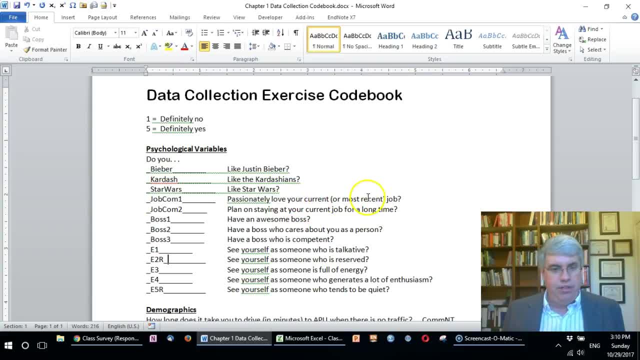 about: do you passionately love your current or most recent job? I called that job comm one for job commitment one. Job comm two was: are you planning on staying in the United States? Are you going to get your job for a long time? And I've got three questions on a boss, And so each question. 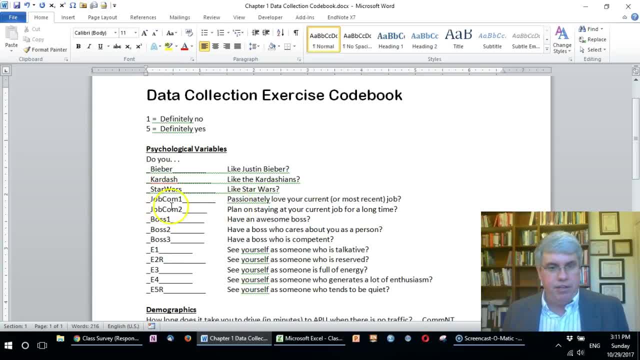 that's measuring the same variable. I've put together Job comm one and job comm two are measuring the same variable. job commitment, Boss one, boss two, boss three are measuring one's attitude towards one's boss. And then I had five questions on extroversion. 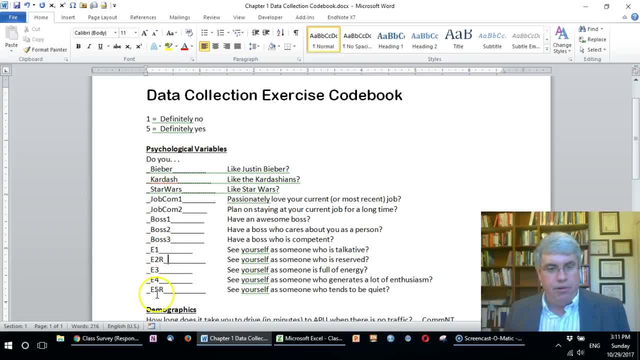 And I labeled E1 through E5. Now some of the questions are reverse scored, And that means so. the first question is: do you see yourself as someone who's talkative? Now, extroverts tend to be talkative, So that's not a. 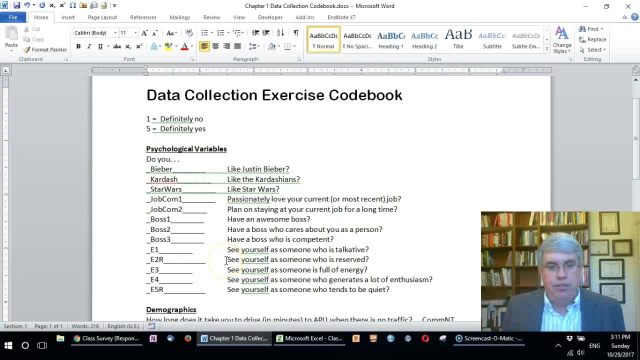 reverse scored question. But then the second question is: do you see yourself as someone who is reserved, So that one strongly agreeing with that giving a high score would be the would indicate the opposite of extroversion, And so this is a reverse scored one. So we need to. 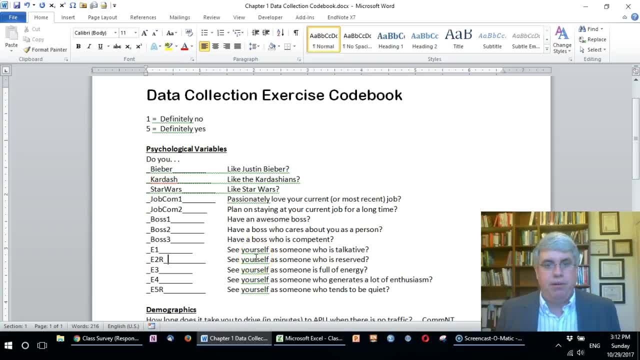 change those scores around later, And there's a separate video on how to do that, But we need to keep track of which items are reverse scored. So the only two reverse scored question items that I have here are: do you see yourself as someone who's reserved And do you see yourself as someone who 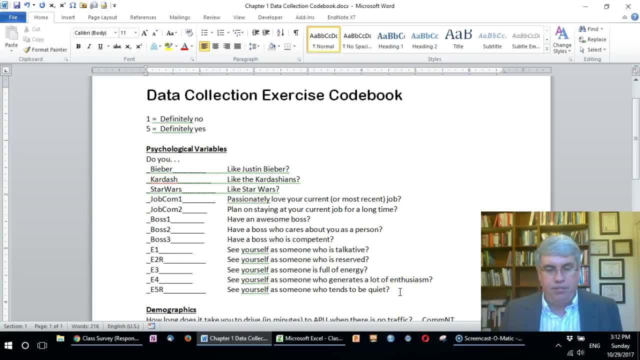 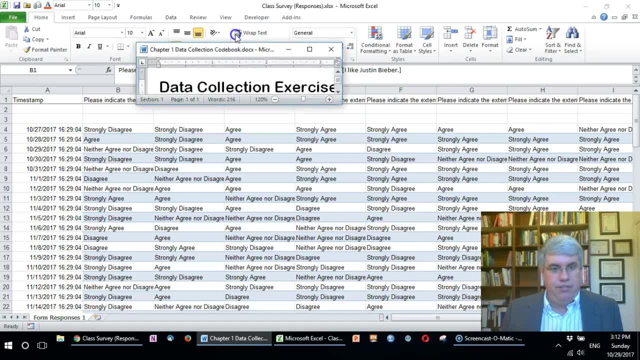 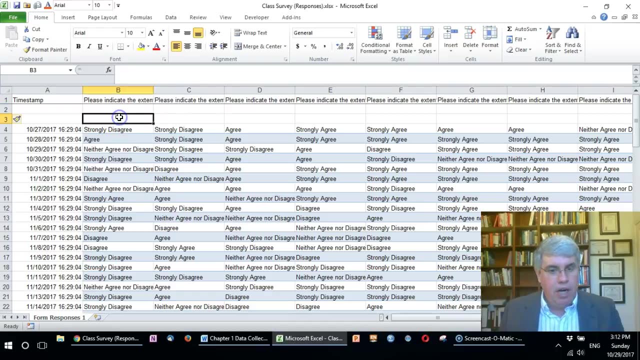 tends to be quiet. Those measure the opposite of extroversion, So they have to. the high scores have to be changed to low scores and the low scores to high scores. So I've got these codes here, And so this first one- I like Justin Bieber, I'm going to call this Bieber, And it's usually best to in. 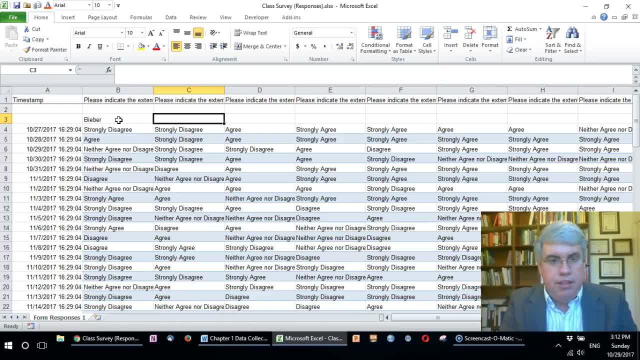 Excel to not have any spaces and variable names. This question, which is about the Kardashians, I like the Kardashians, I'll call that Kardashian. The next one is on Star Wars, Making them all one word, with no spaces. So this was. I passionately love my current job, So this: 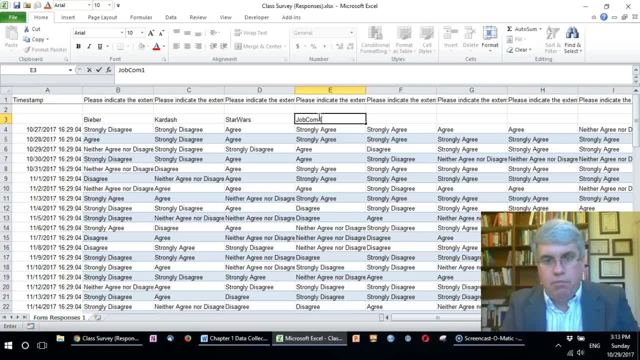 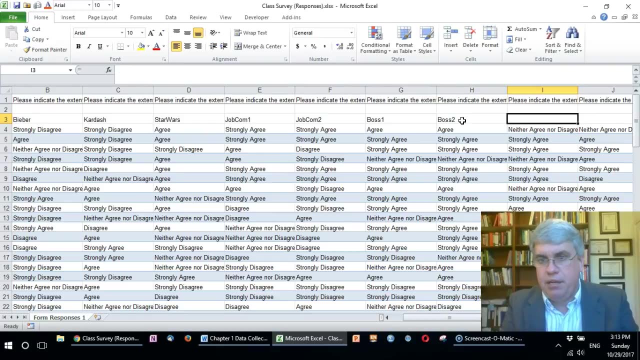 is going to be job com one, The next one's job com two. Now, it's super important not to make any mistakes about these. Here's boss one, my attitude towards my boss, Boss two and boss three: I can use tabs to go from one cell to another, And I can also use tabs to go from one cell to another. 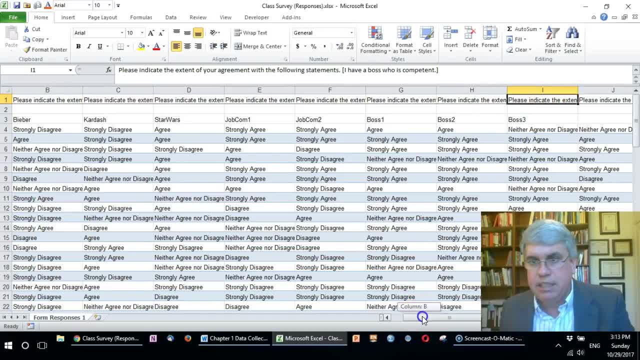 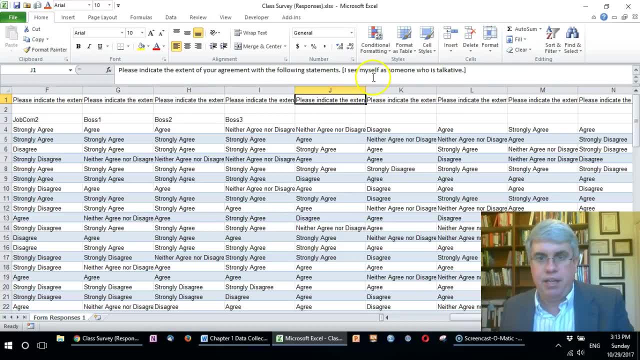 Easily So, boss. three was: I have a boss who's competent, Let's move over a little bit more. So the next one is: I see myself as someone who's talkative. So this is E1.. Now, something important is that all the I've got five extroversion questions and we said some are reverse scored. 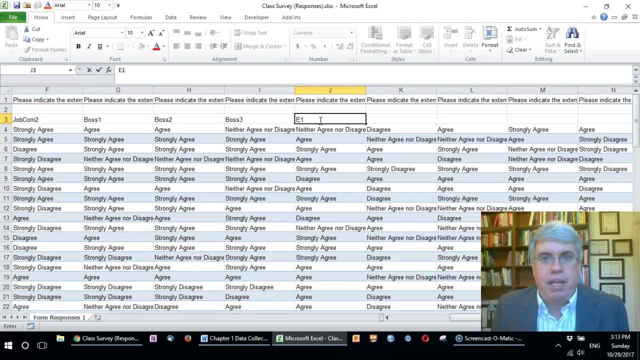 but sometimes there's subscales when you measure something, And so if we had different subscales of extroversion, like you might want to measure extroversion dominance or extroversion sociability, because they're both associated with being an extrovert, Extroverts tend to be dominant. They 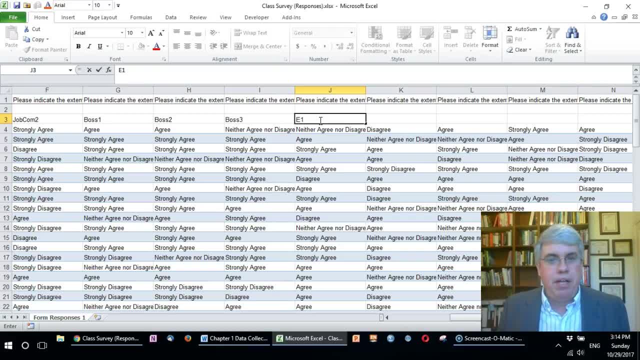 tend to be sociable. But you, there are different subscales. So we, if this had been a dominance question, I could call this EDOM1.. And if there was a sociability, I could have called it ESOC1.. I knew that both at start and end, I could have called it ESOC1.. So I knew that both at start and end, I could have called this ESOC1.. So I knew that both at start and end, I could have called this. 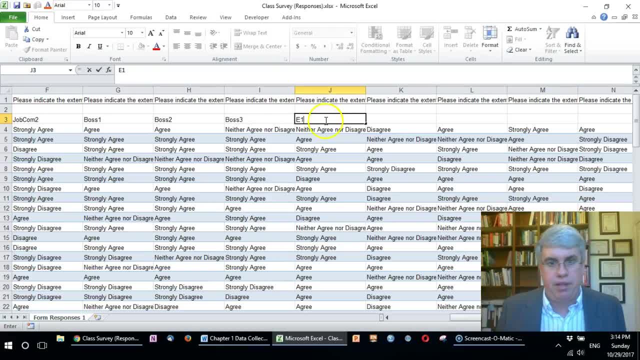 ESOC1.. I knew that both at start and end I could have called this ESOC1. So if I have to start with, E would be extroversion. But I clarify what subscale they belong to: A subscale they belong to. So this was. 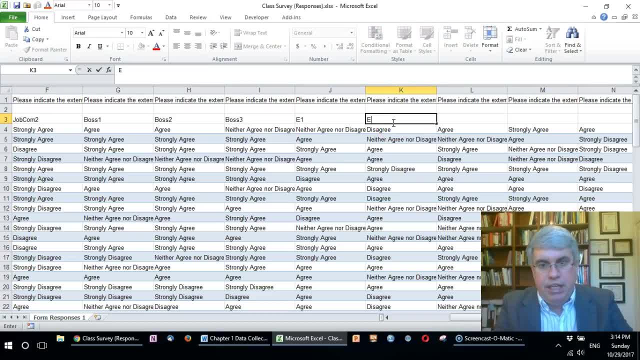 I see myself as someone who's reserved. This is E2. Now, when we unreverse it, eventually will just call this E2.. This one's E3,, you've got E4.. And then, finally, we've got. I see myself who is someone who tends to be quiet. That's E1.. 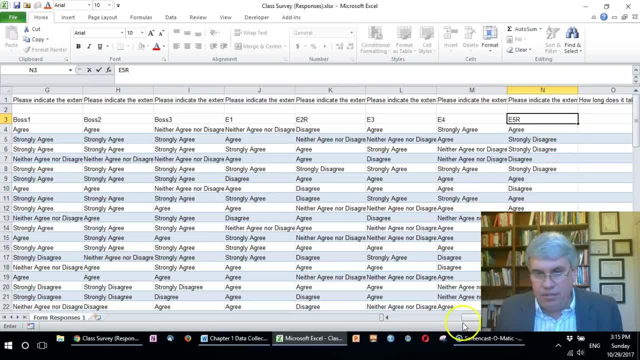 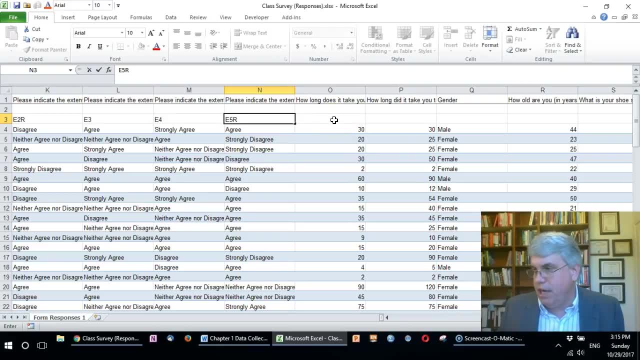 five reversed. okay, let's slide this over a little bit more. now. we've got some questions about commute time and on my X, the code book. this first one: how long does it take you when there's no traffic? that was I called that one. look on to my code book: commute, no traffic. and then this one is: 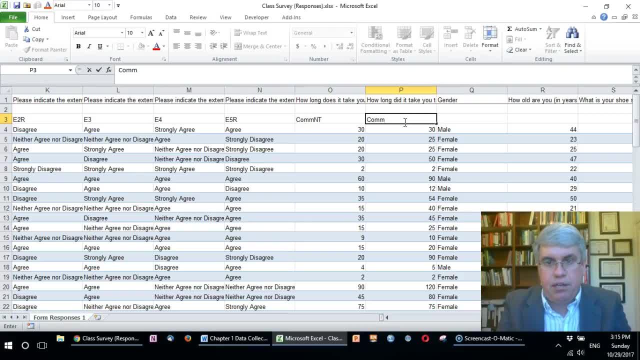 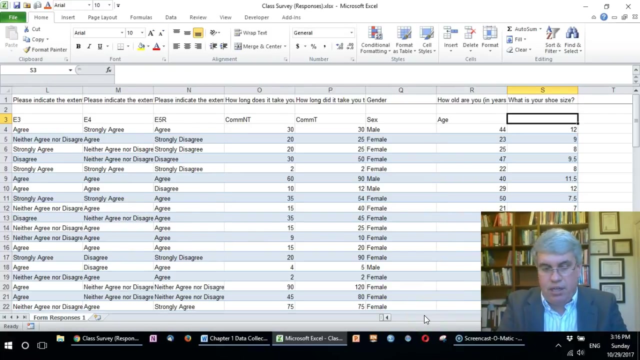 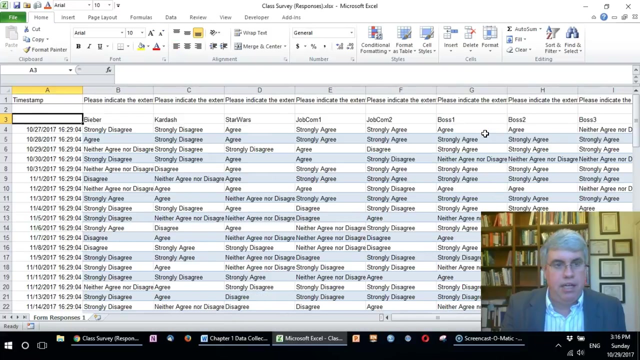 commute with traffic, which are called cmt. now here we've got sex or gender. you can do either one, as long as you know what the numbers are referring to. how old are you in years that one will be age, and then our final question is: what is your shoe size? and I'll just call that shoe all right. so now we have names for. 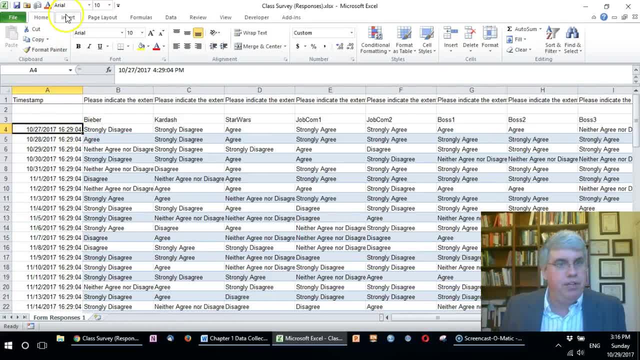 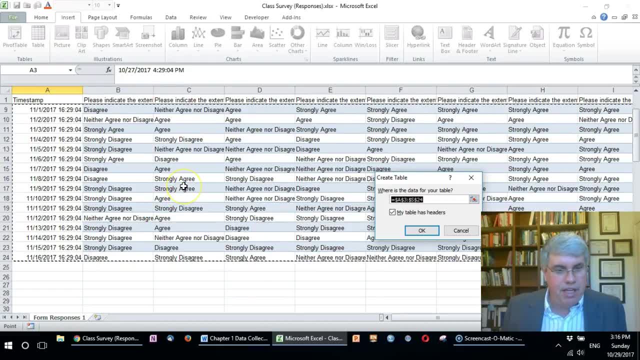 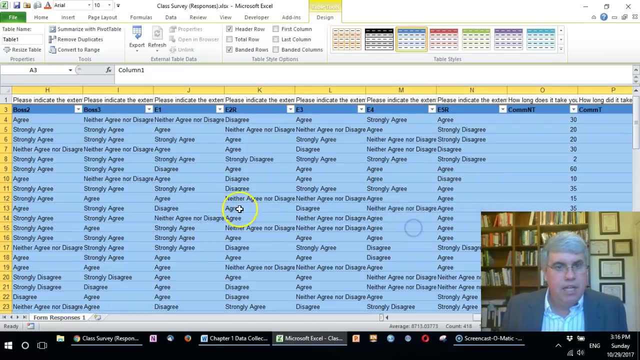 all of our variables. let's put this into a table. I'm going to do insert table and it says: it's this what the table is supposed to be? and it looks like it is, so I will go okay. and now we have the variable names and we can sort by those variable names if we need to now, before we can, 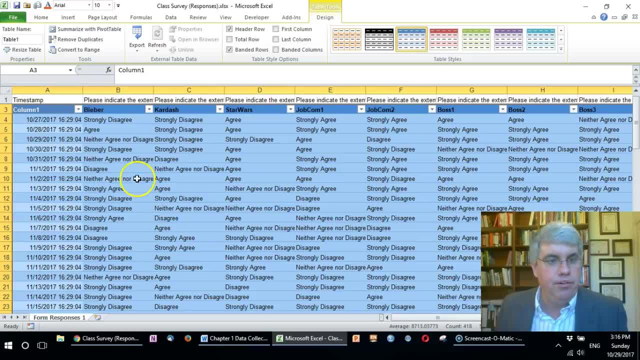 analyze. another important thing that we need to do is we need to change all of these: strongly disagree, strongly agree, agree, neither agree nor disagree. we need to change all of our variables. so, for example, my name is naney, i support, my student is naney. we're going to do part two of the 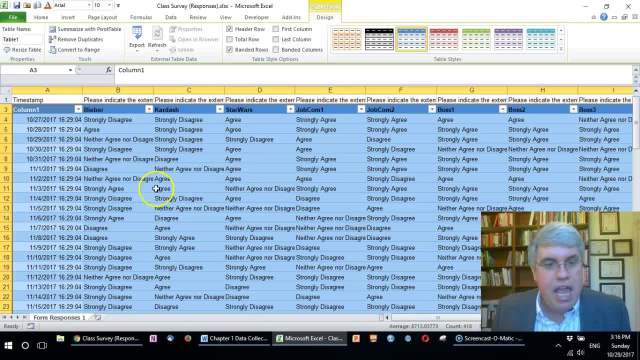 this to numerical values, and this is a little tricky because you can't just say: oh, let's go replace all the words agree, because that occurs in agree, strongly agree, slightly, agree. if you use that, disagree even has the word agree in it. so what we need to do is we need to start with the longest phrases first. so 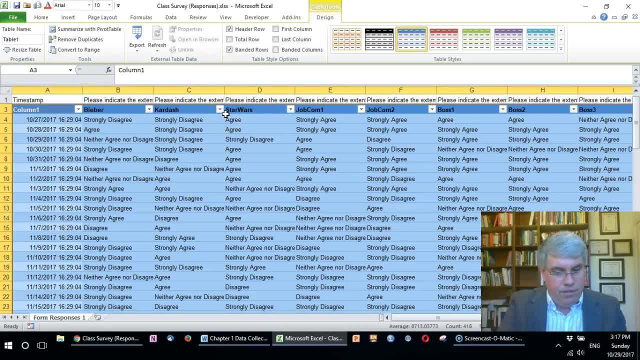 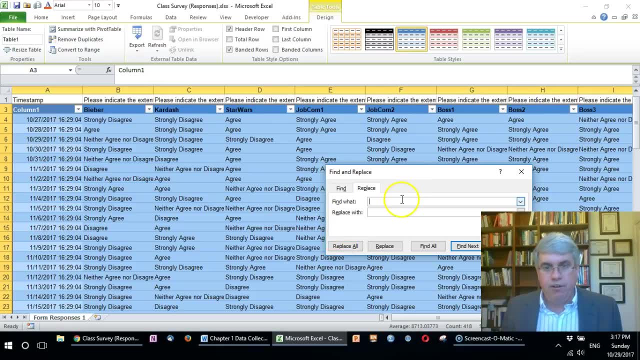 we're going to go to. let's go to do ctrl F for find and we want to choose the find and replace. and the first thing, the longest one, is: neither agree nor disagree, and that is our middle value. let's let me bring the code book over. 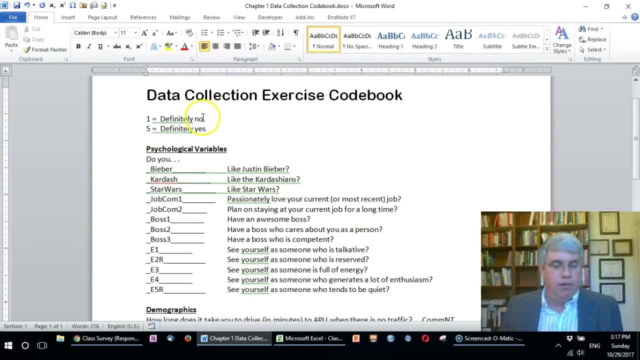 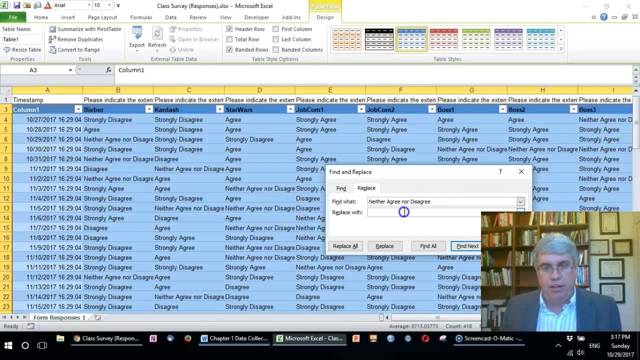 here, and one was a definition of the word agree and the other one was a definition of the word disagree, and that is our middle value. let's let me bring the code book over: definitely, no or disagree. five was a definitely yes or strongly agree. so then, neither agree nor disagree is our middle value, and we're gonna replace 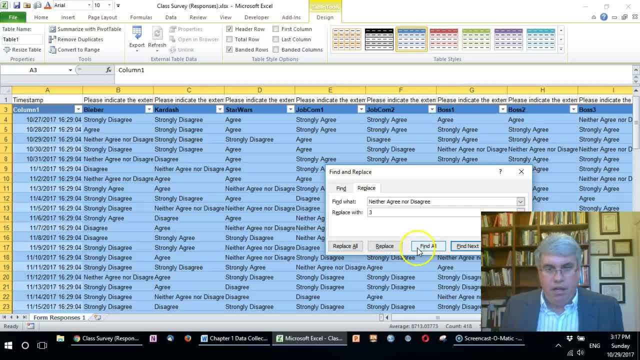 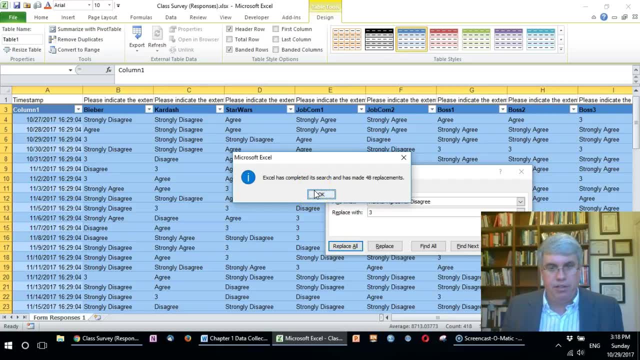 that with three, so let's replace all. and so there were 48 places that people had marked the neutral value there. neither agree nor disagree. now let's look for the, the next longest, which would be string, strongly disagree. so I change that to strongly disagree and that's going to. 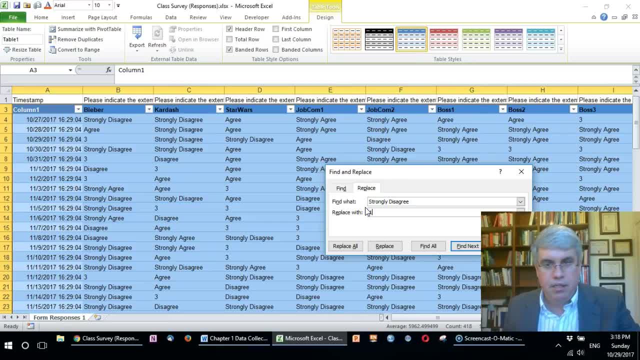 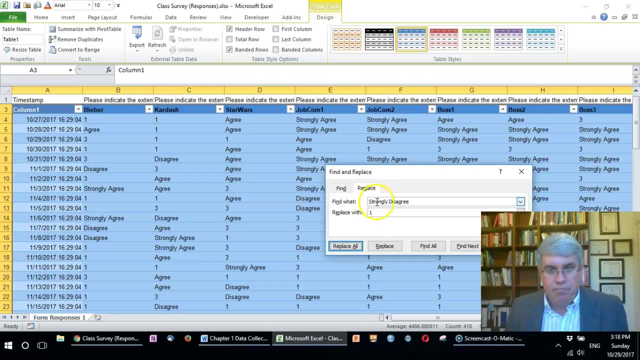 get replaced with a one, because strongly agree is shorter than strongly disagree and we want to start with the longest ones first, strongly disagree, which is the first value, the lowest value, and replace all. okay, so that got rid of a lot of them. now we're going to go to strongly agree and I've got a capital. 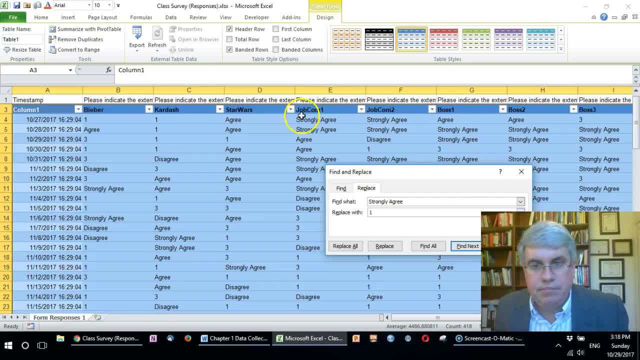 capital A and the way that I designed the, the survey, and we're going to replace that with a five. replace all, okay. now we're gonna. we've got disagrees and agrees left. let's replace the disagree, and that is a, to the second lowest- replace all, okay. and then we've got agree, that agrees, let's go to the second lowest and then we've got a degree that. 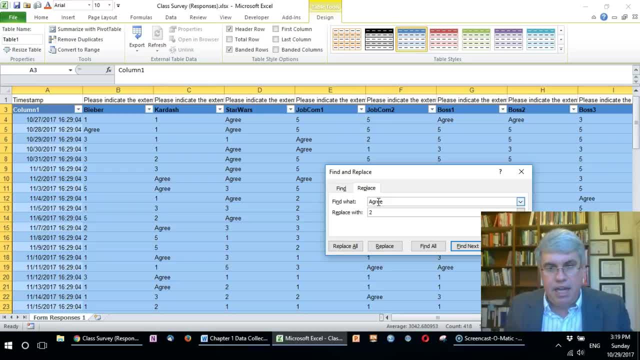 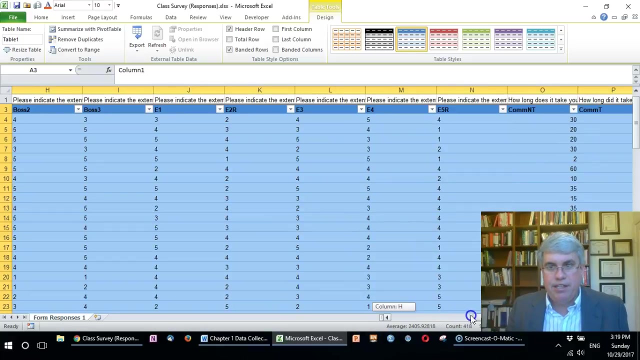 that is left and that's going to be a four. Now, if I made a mistake any place along the line, I could use control z to undo my mistakes, So let's replace all. All right, so we have replaced the words with the numbers, except if we go over here we find that, oh, we've still got a few. 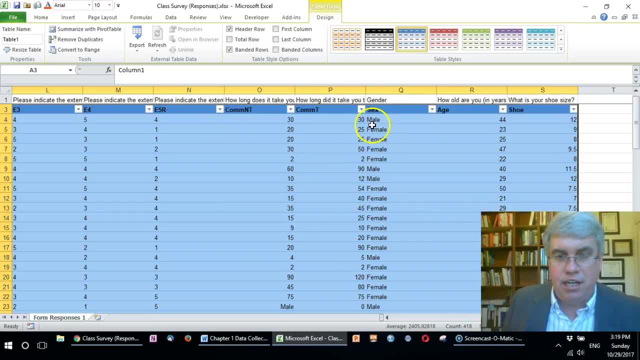 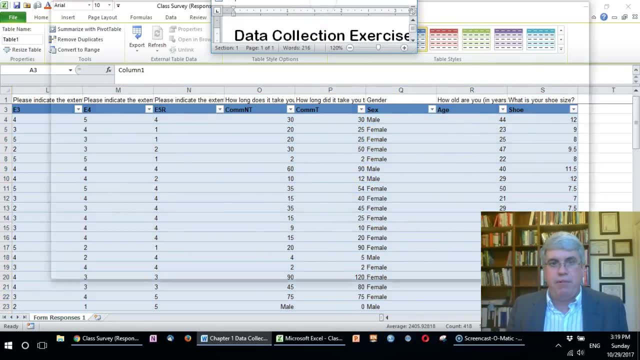 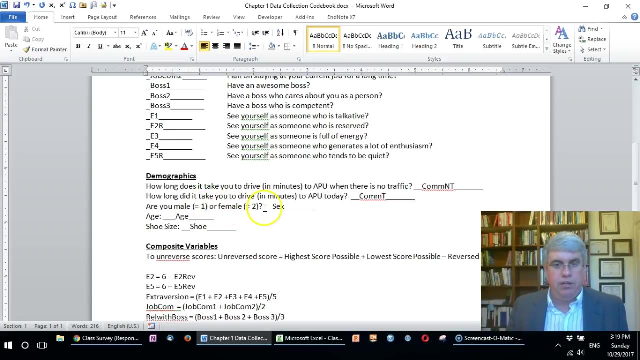 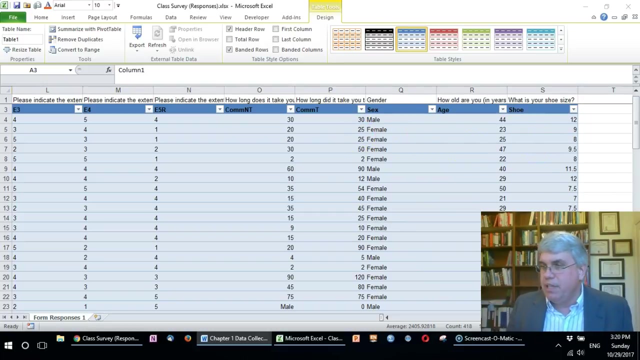 things. We've got the sex that is labeled male or female Now in our code book and the way that we asked the survey we specified: are you male or female? One or two. Now asking if you are male or female, that's kind of it's not clear if that's sex or gender Sex usually. 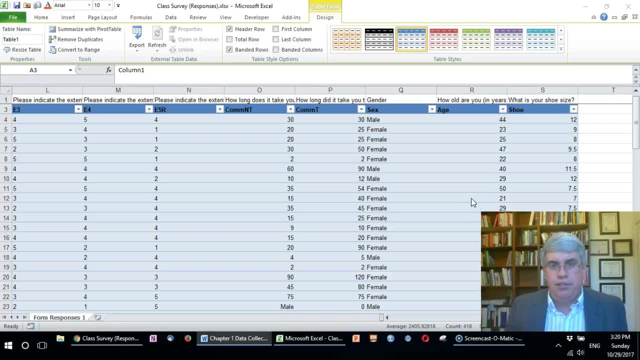 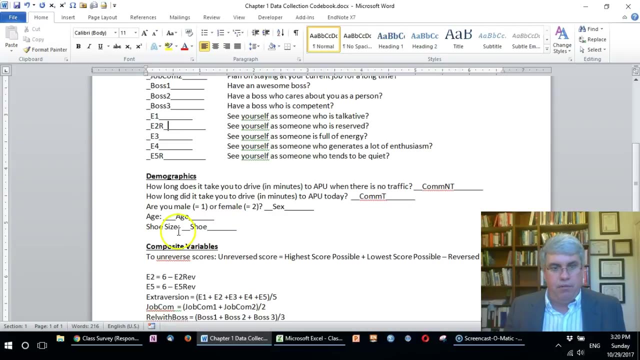 refers to one's biological state, and gender usually refers to one's self-perception. We only gave people two choices, so they probably viewed that as a sex question- male or female- And in the survey we had said that one was male and twos were female. So that's what we will convert this. 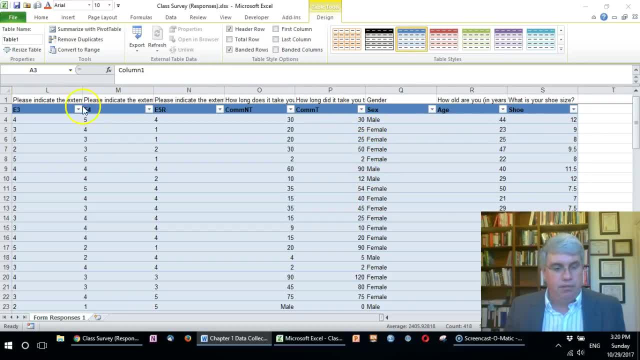 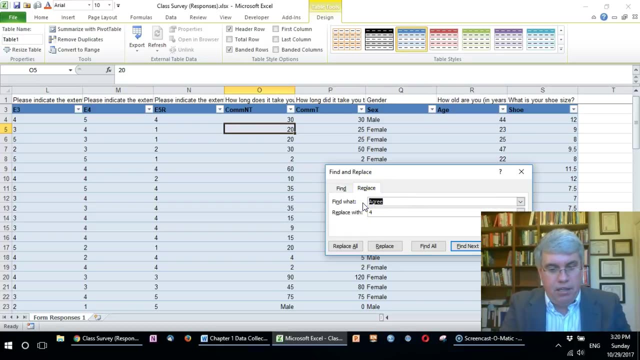 as. So once again, we want to start with the longest, So we're going to do control, find. wait, let me click in the right cell here, or the right program. So control, find. I'm going to choose, replace. Let's choose female, which we said was two, Replace. all Okay, now let's go for male. 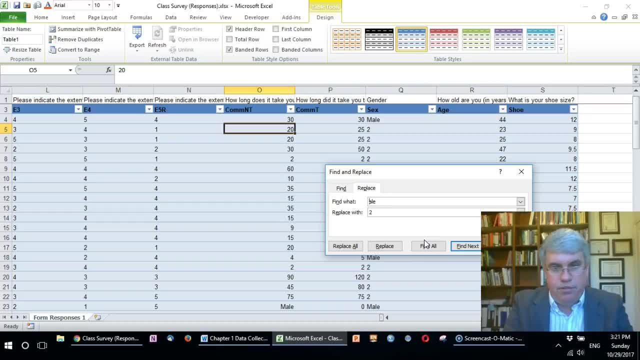 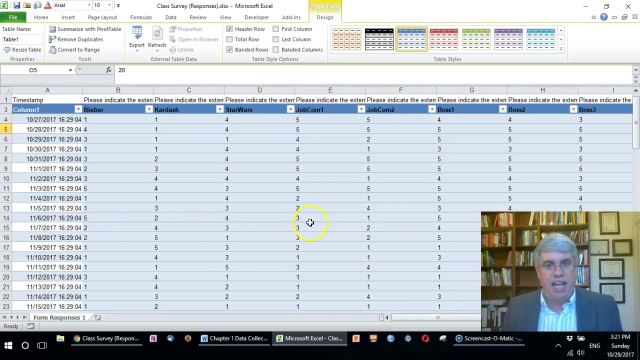 which is the shorter of the two, and replace that with one, And there we have. all of our data is now in numeric content. Now is there anything else we want to do to replace, to prepare this data before we start analyzing it, before we check? 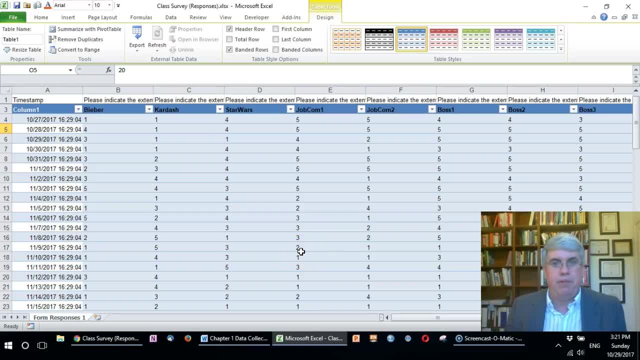 clean up the data to see if there's any bad data in it, or before we start making our composite variables. This first column, the timestamp. we don't really need that, but sometimes it's nice to have that in there. So let's go ahead and do that. So let's go ahead and do that. So let's go. 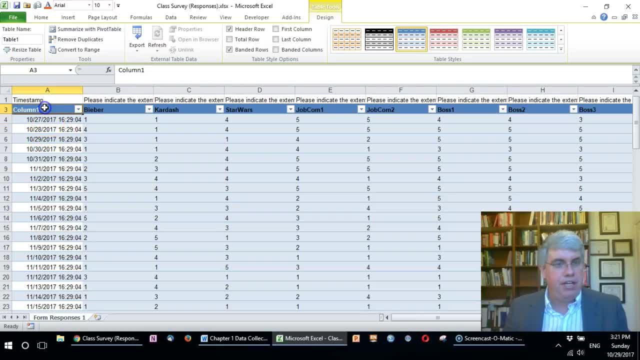 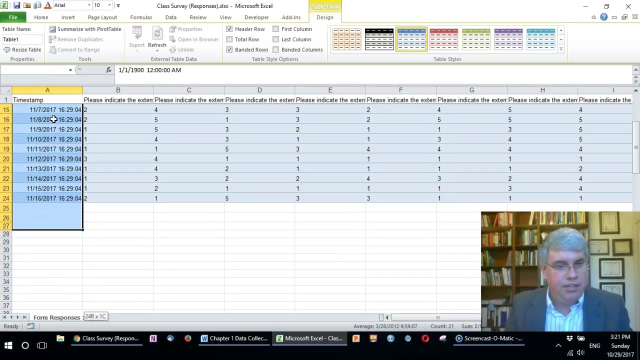 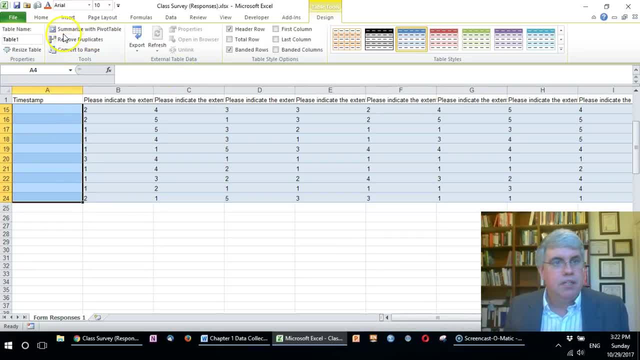 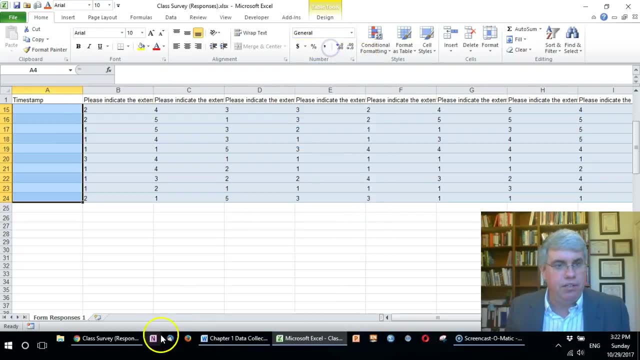 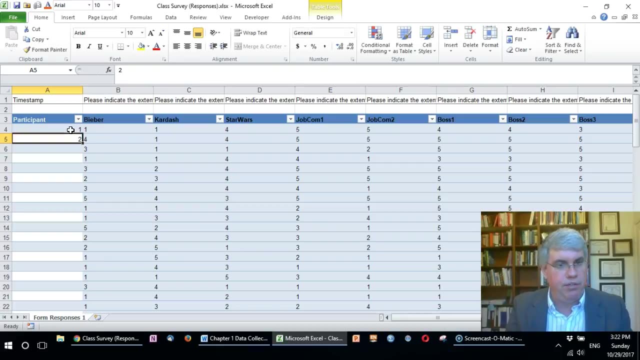 delete everything in there, Delete. Let's go to home and change that to the format. Let's just call it general, no specific format. participant. we're gonna call the first one, one, the first one, two, second one, two. now what we can do in Excel, if I do go up to the top one, press shift down arrow. 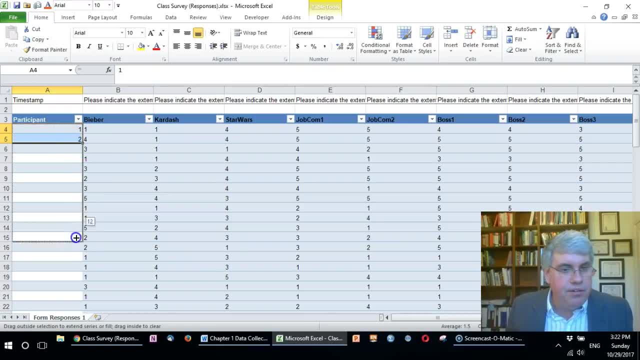 select those two. I can just drag this all the way down to the bottom and I get a number one through 21. so we can, we can. I'm going to change this to participant number so that if we want to talk about participant 9, something like that. so now, 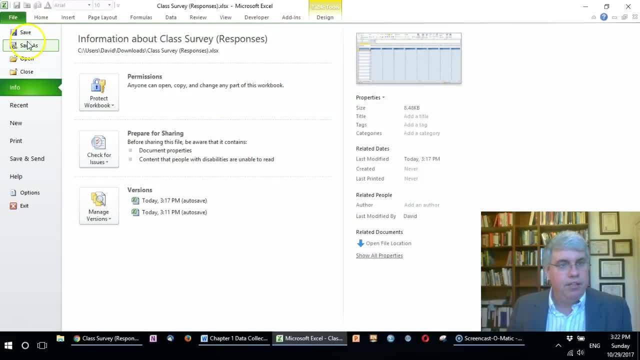 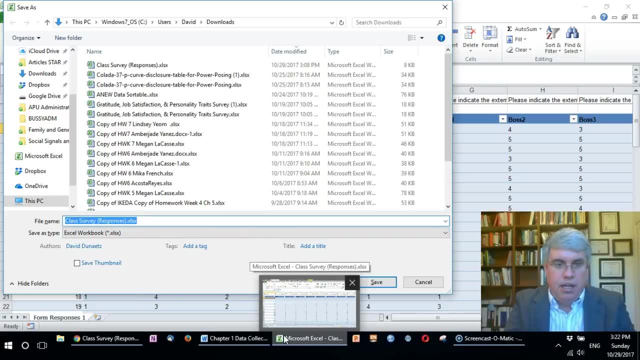 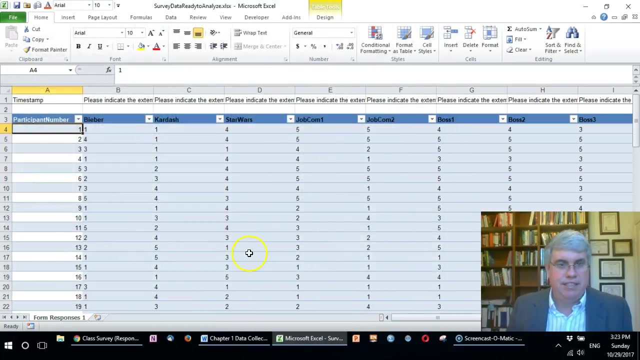 we. we better save this to file, save as- and we will call this survey data ready to analyze, and I should have done that at the beginning, because it's horrible to lose your data and lose your work at the after. you've been working out for a while, so now we've got survey data ready to analyze in an Excel spreadsheet. 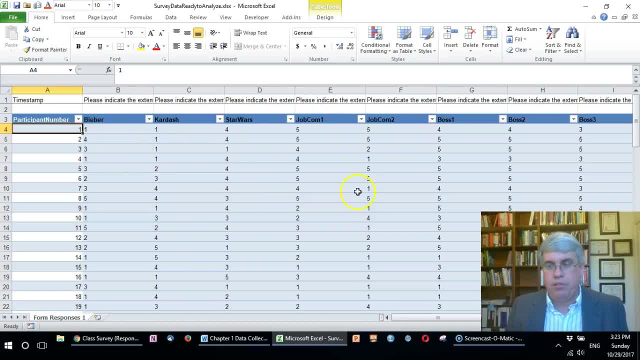 format in call, with columns, with the variables clearly identified, and now we can go and clean up the data and then create our composite variables after we convert the reverse script. and then we can go and clean up the data and then create our composite variables after we convert the reverse script. and then we can go and clean up. 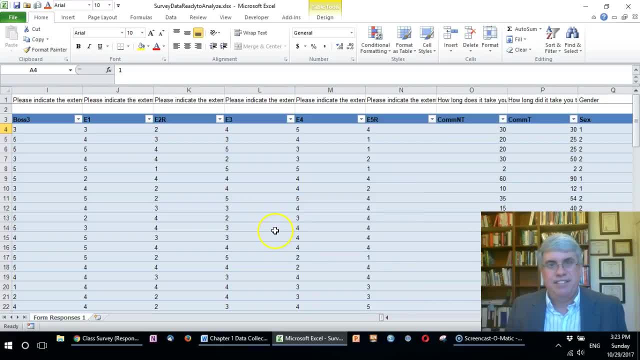 the data and then we can go and clean up the data and then we can go and clean up our composite variables quickly organized. we have to switch over. so this is the our composite variable, quickly organized. we have to switch over. so this is the 76 Paige you.